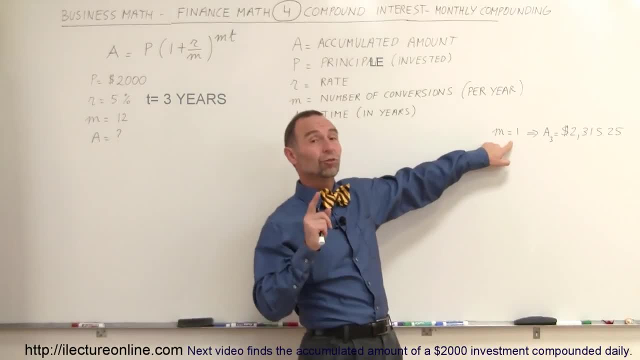 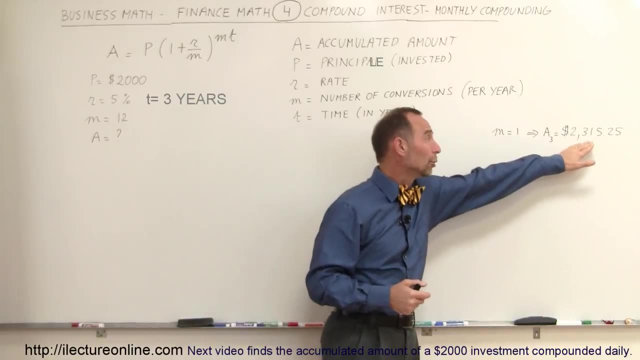 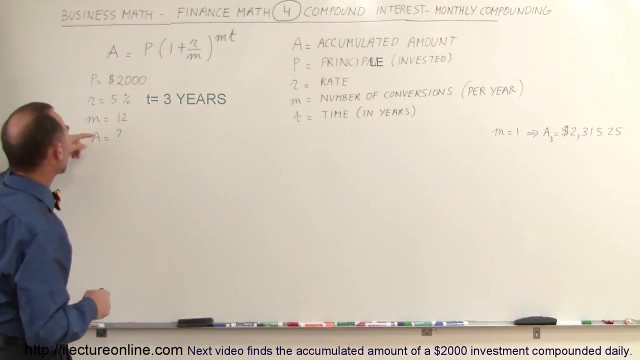 In the previous video we showed that if the number of conversions per year is one, meaning we compound the interest yearly on the $2,000 investment for three years at 5%, we would earn $315.25 of interest. So let's see how much more you would earn if you were to compound monthly. 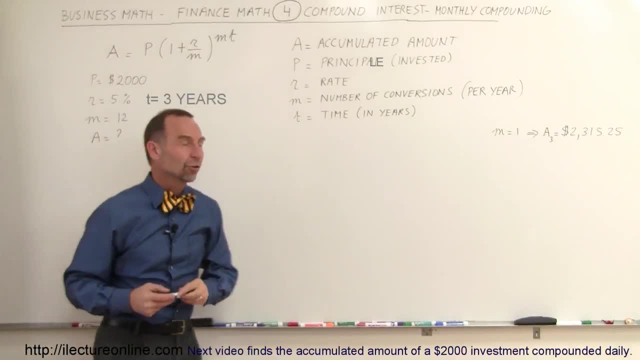 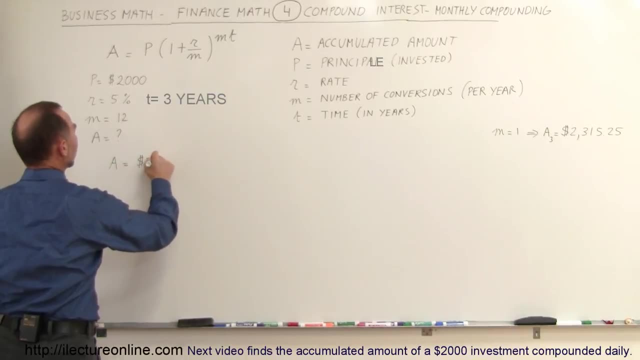 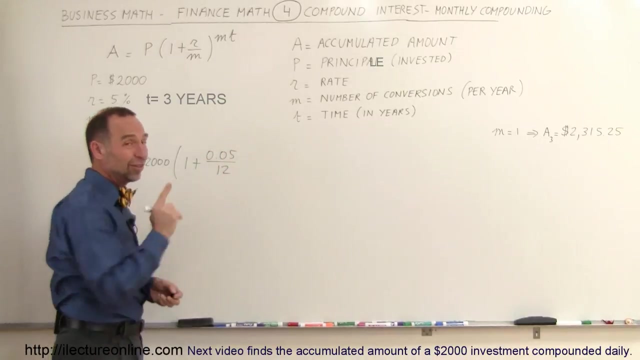 So here m is going to be 12,. m is, of course, the number of conversions. There's the equation we use. So the amount accumulated after three years is equal to the principal invested, which would be 2,000 times 1, plus the rate 0.05, divided by the number of conversions. So in this case, 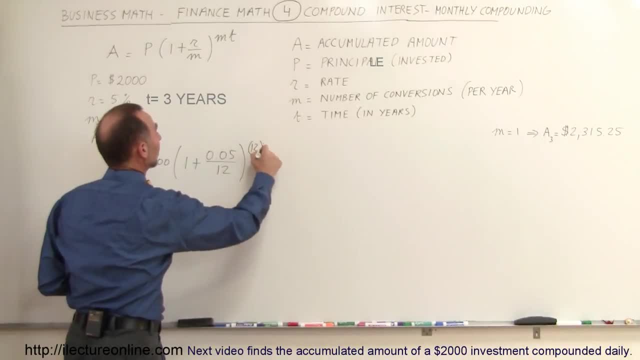 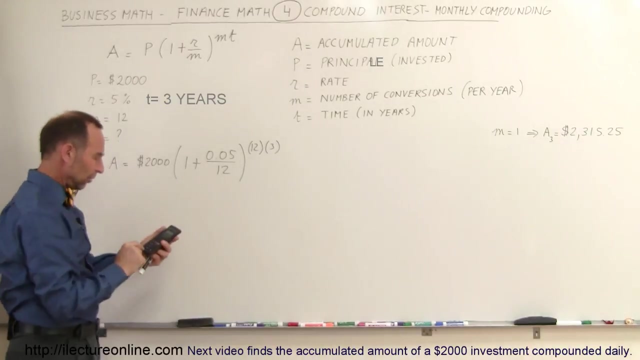 monthly would be 12, and then you raise that to 12 times t would be then, of course, three years. So we raise that to the 36th power. Okay, so you can see why you'd want to use a calculator for that. So we get 0.05 divided by 12.. I work from the inside out So that I add that to 1, and then 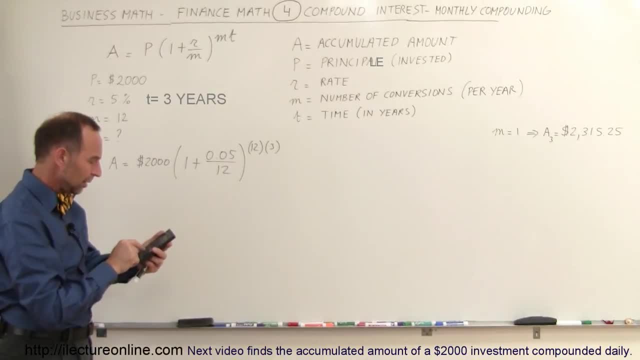 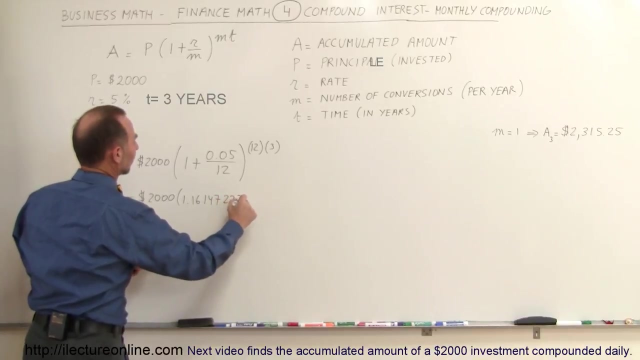 the 36th power. So I find my x to the y button 36.. And so then you end up with: this is equal to 2,000 times the quantity 1.161472231.. Of course, do we need all those figures? Not really. 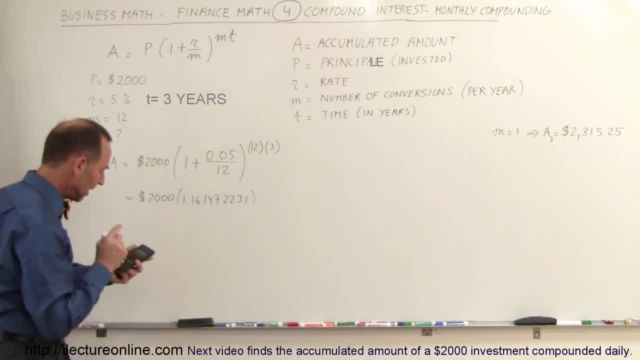 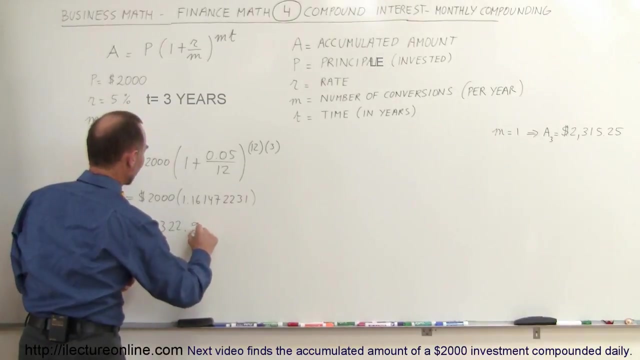 but I just want to show you that if you use your calculator, you should get something very similar to that. If we then multiply the times 2,000, we get a total amount accumulated, a to be equal to $2,322.94.. So we usually round that to the nearest penny. Now notice the. 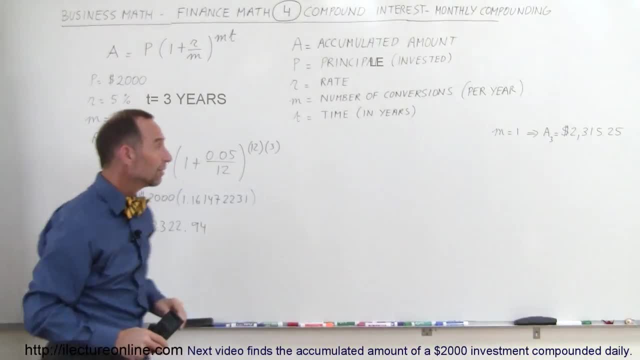 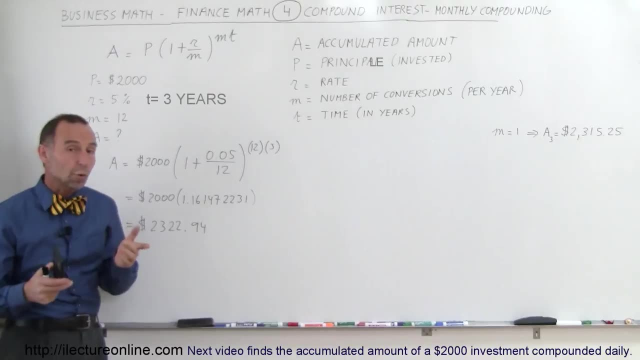 difference. So there was only $315.25 of earnings. Here would be $322.94 of earnings. So we'll earn about $7.5 more compounded monthly versus compounded yearly. So you can see it wasn't a lot of dollars, but it sure was a nice advertising. 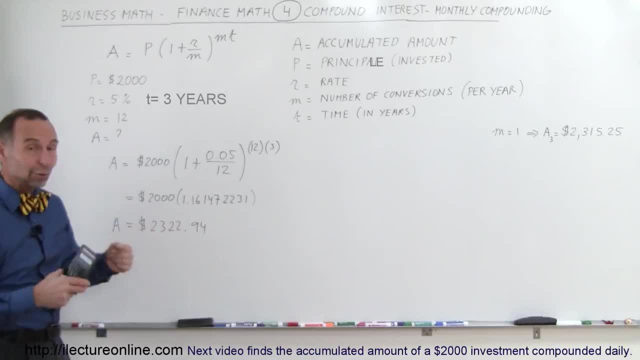 Stunts for those banks who were willing to calculate every month, they could lure in customers claiming the customers make more money. Of course the difference between $315 and $322 isn't really a lot, but the psychological effect is: look, we compound more often.